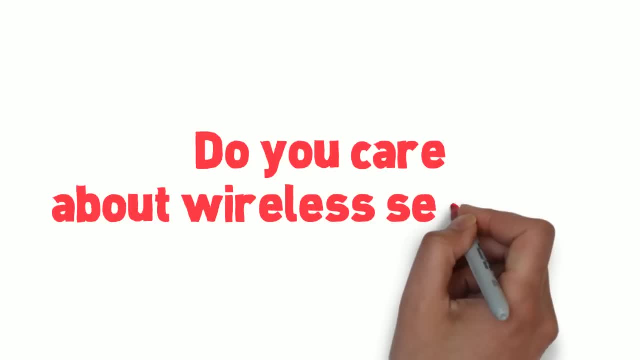 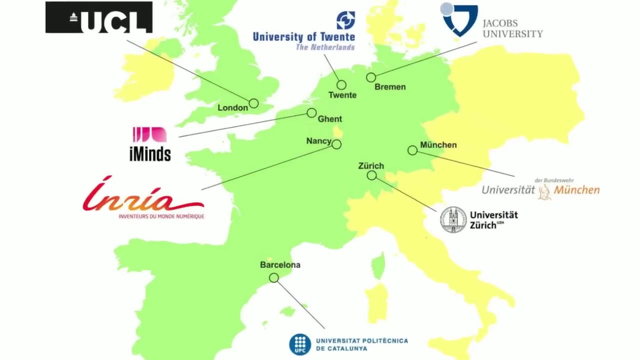 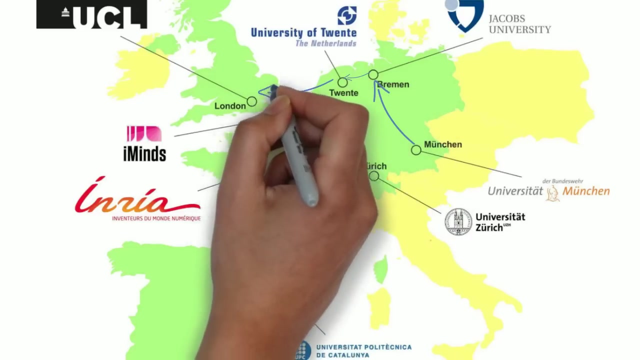 Do you care about wireless security? Why is wireless security an important topic? You all know the situation when you're traveling around for project meetings or conferences. Imagine several collaborations where researchers work together on specific topics in the area of network and service management, like in Flamingo. 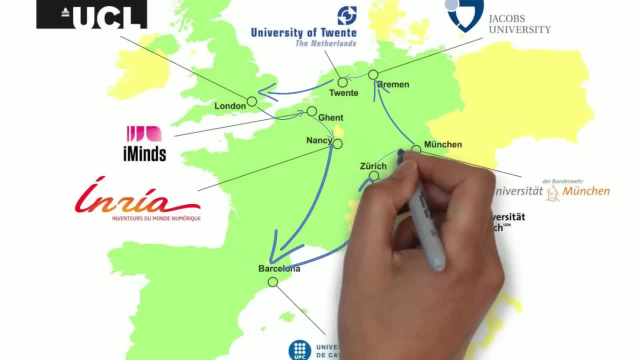 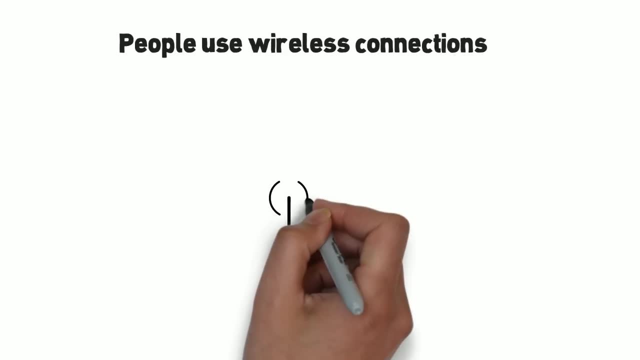 They meet at several locations of their partner universities. Nowadays, you can find everywhere a possibility to connect to the internet. Since more and more devices are equipped with a wireless interface, this is possible without any additional hardware involved. You can get connected with your mobile. 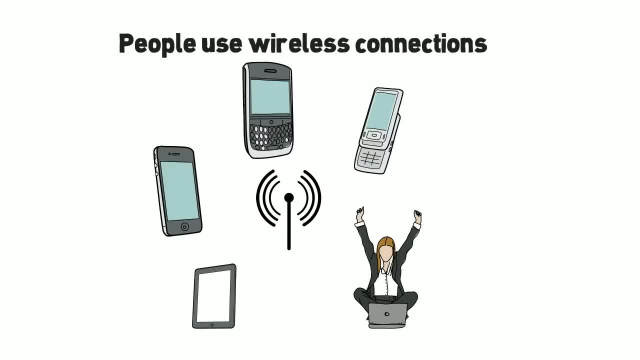 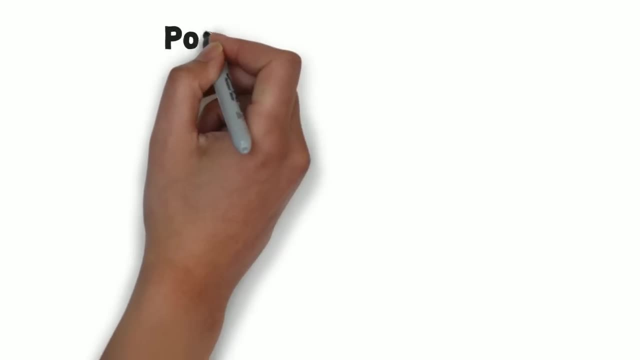 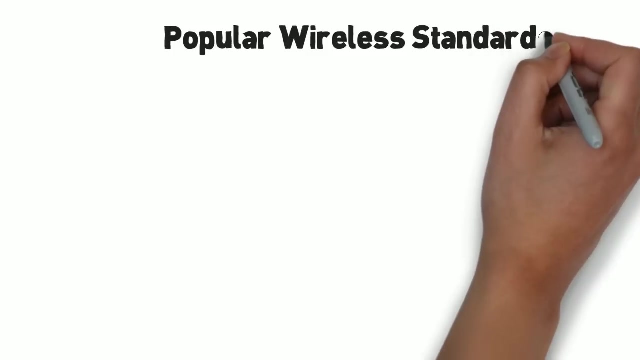 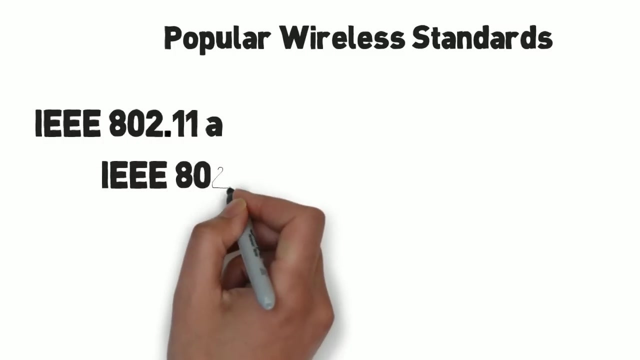 your blackberry, your laptop or your tablet device everywhere. Almost all public available devices are equipped with an interface which allow a connection to wireless networks. Therefore, several standards exist to allow an interaction between different manufacturers. The most popular standard is IEEE 802.11. 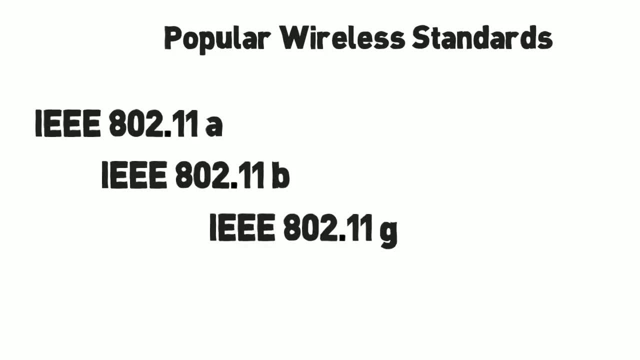 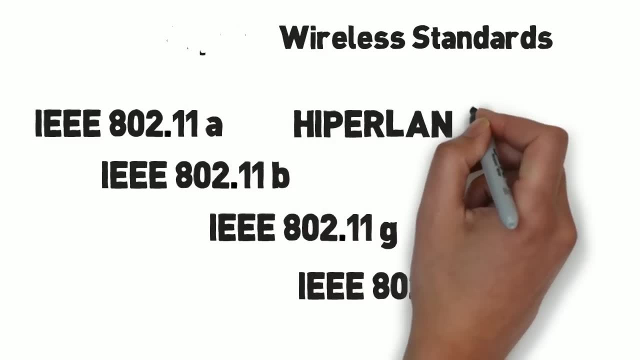 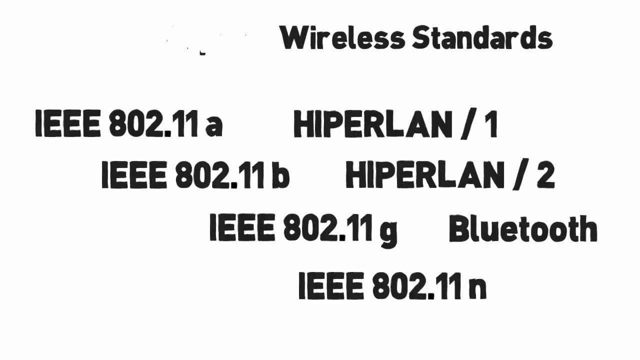 with its specifications A, B, G, N. Besides these, there exist standards like Hyperland 1 and Hyperland 2, Home RF or Bluetooth, where only the latter one is important today in transferring less amount of data. Now let's think about the security. 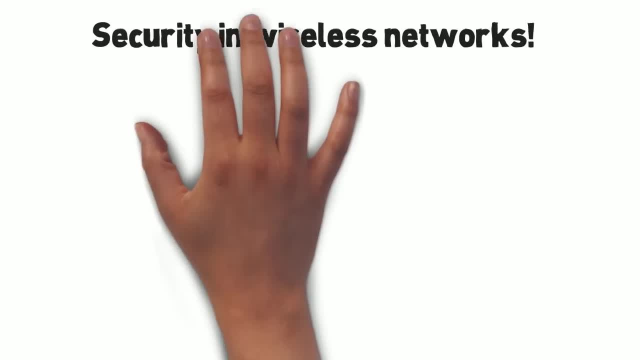 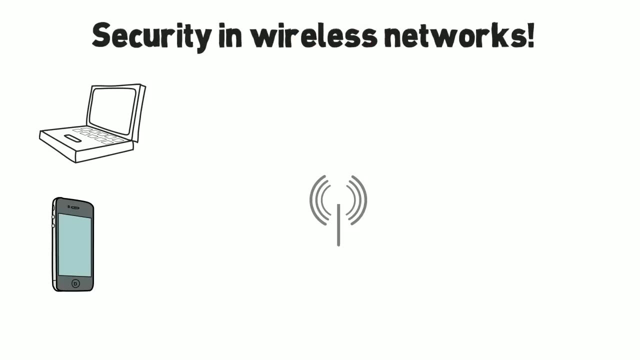 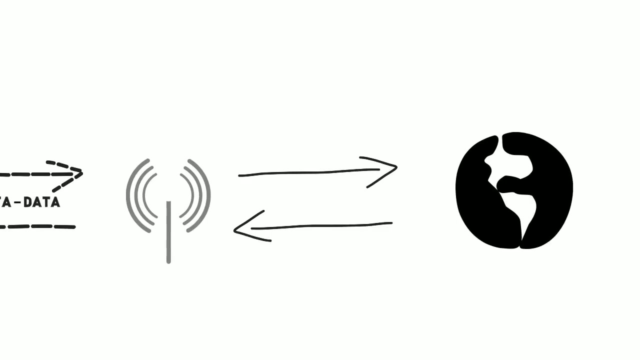 in such a network where no physical security is possible. Imagine the following scenario: A laptop or mobile tries to get connected to the internet via a wireless network. Do you see any attackers in this scenario? Have you ever thought about possible endangerments regarding the wireless connection? 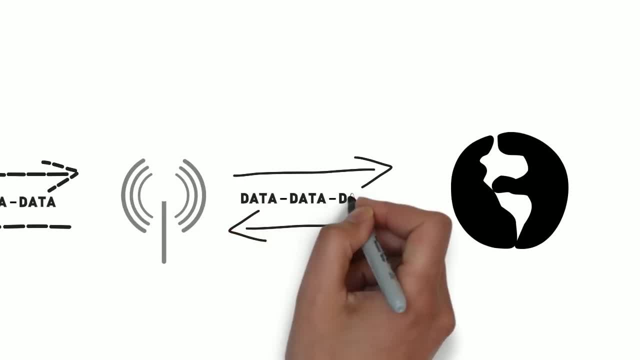 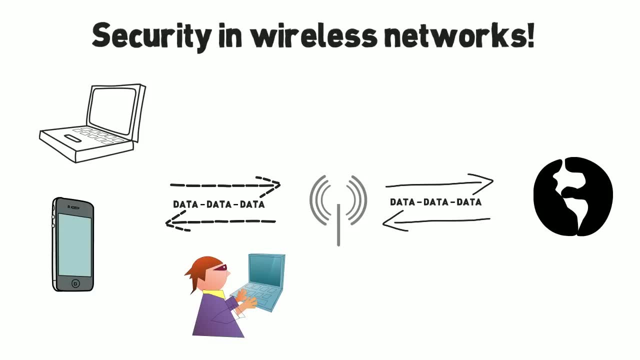 Do you know who can access the data which is transferred from your end device to whatever services you are using? Remember, none of the aforementioned standards, except the Hong Kong standards, do not offer Bluetooth. describes security aspects within a wireless network. Do you feel safe in this situation where an attacker plays man-in-the-middle to catch your 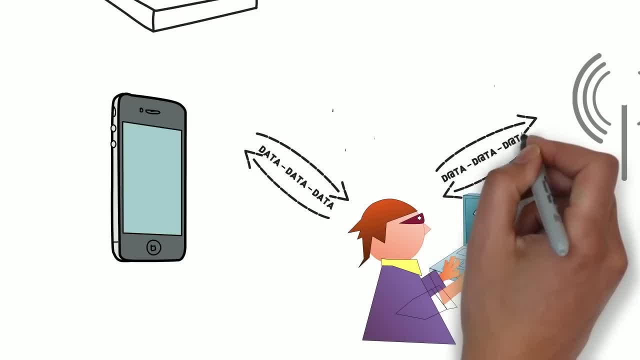 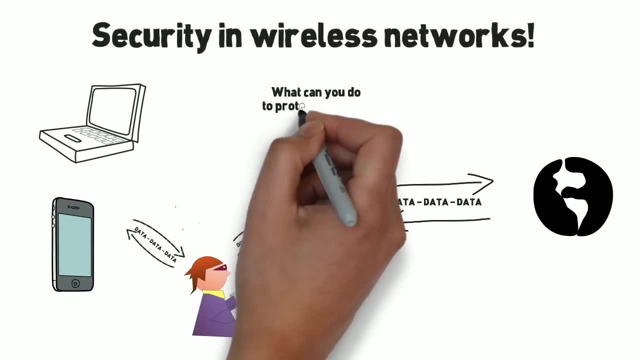 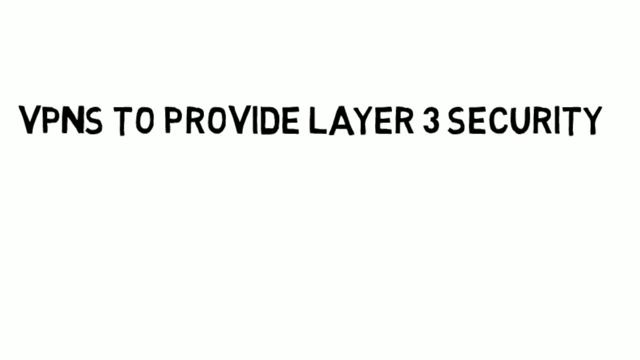 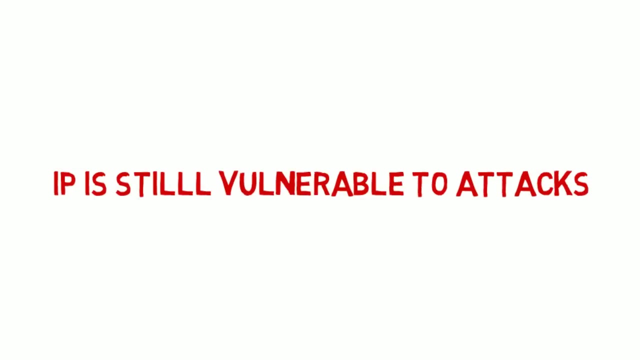 data, hack your bank account or does other criminal activities? How to secure wireless connections. Security has long time been the trade-off within Wi-Fi. Early wireless networks leaned heavily on VPNs- virtual private networks- to provide a layer 3 security which left the IP network vulnerable to attacks. 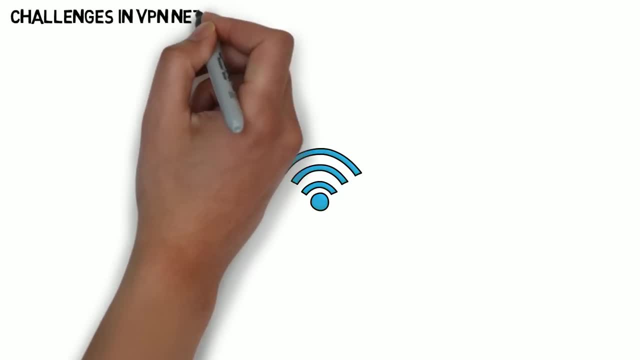 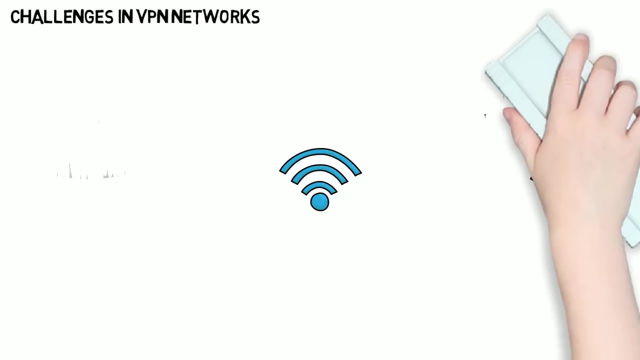 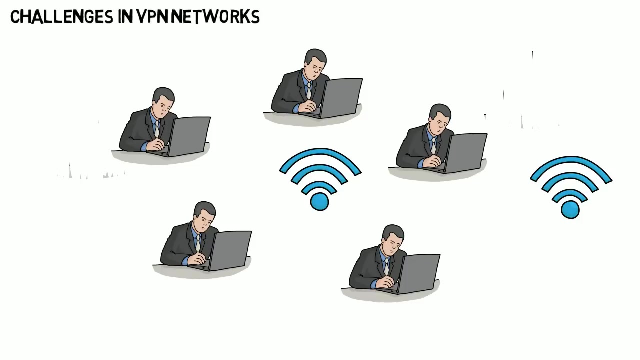 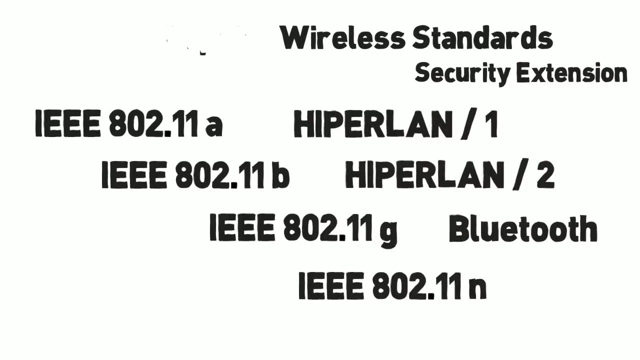 In addition, it introduces several challenges. The first to mention is roaming, where you travel with your connected device from one to another access point. Others are quality of service, client support or simple scalability issues. within this case, Therefore, security extensions were developed to allow the establishment of. 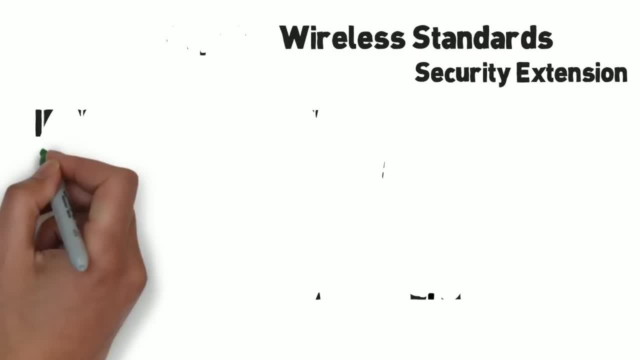 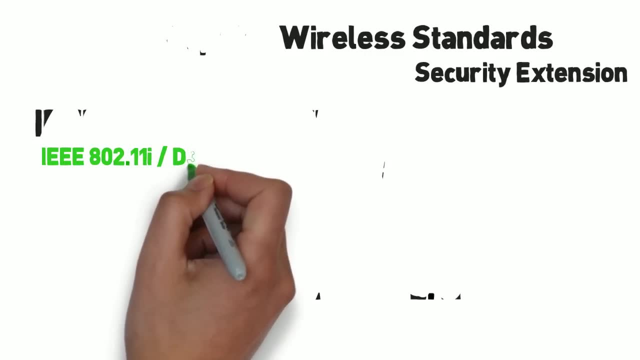 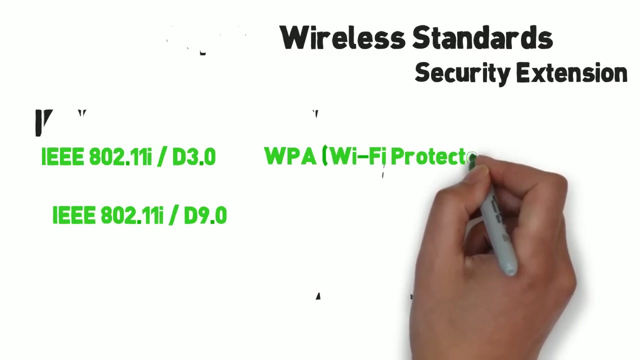 security mechanisms. IEEE 802.11i D3.0 and IEEE 802.11i D9.0 are commonly known as Wi-Fi Protected access- WPA and Wi-Fi protected access version 2, are commonly known as Wi-Fi. 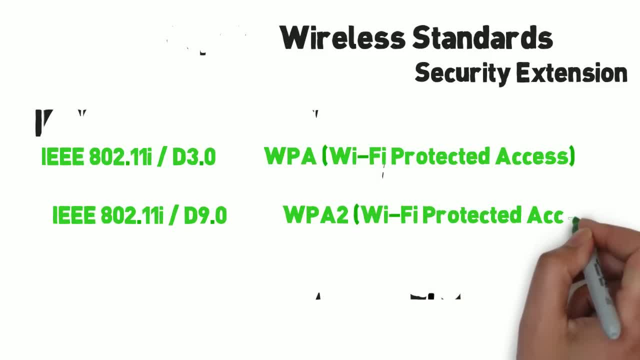 Protected access WPA and Wi-Fi: protected access version 2, are commonly known as protected access WPA and Wi-Fi. protected access WPA and Wi-Fi. OK, now you can use the language you like. This is what's in text text copy. text copy. text copy and text copy. It's an important. 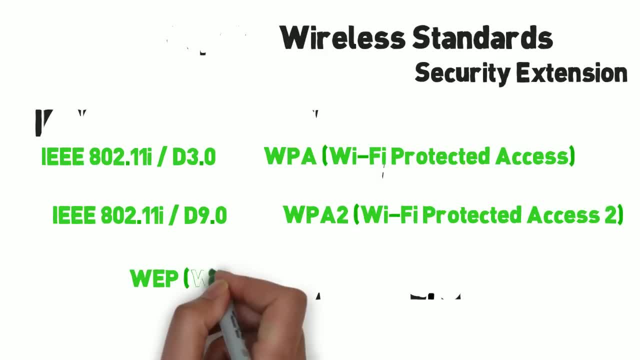 WPA2, the former security extension Wired Equivalent Privacy, is still existing but not secure nowadays. The WPA2 specification is a major improvement over WEP, which has the former security standards of IEEE's original 802.11.. It was susceptible to attacks and poorly implemented by vendors. 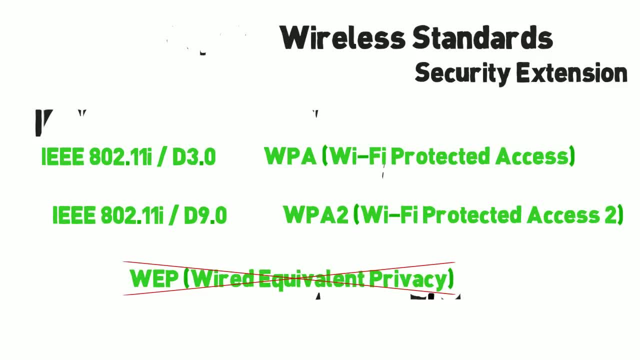 These weaknesses and the ease with which they have been exploited led to the 802.11i standard, which was approved and published in 2004.. The Wi-Fi Alliance created WPA as a subset of 802.11i, 802.11i and later WPA2, which provides stronger security than the first version of WPA. 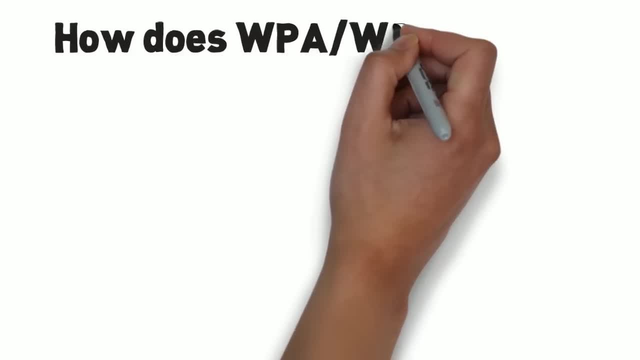 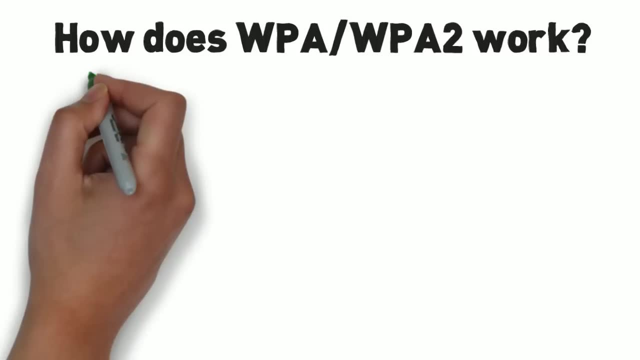 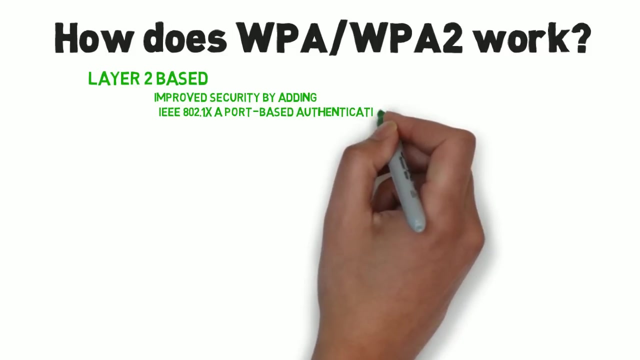 So how does WPA and WPA2 work? WPA2 protects the network better because it is a Layer 2 based, But WPA2 alone can't provide enterprise security. Most security concerns, Most security concerns, can be eliminated by combining WPA2 with IEEE 802.1X, a port-based authentication protocol for access control. 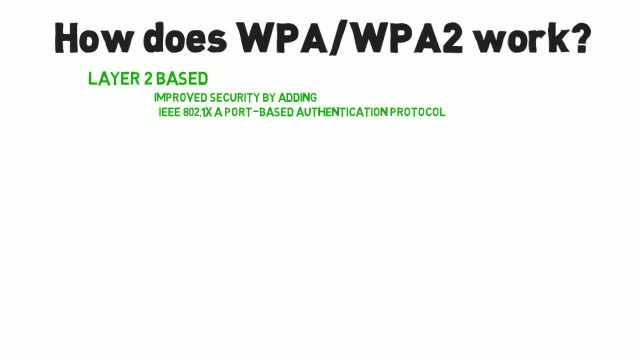 Interference rogues and denial-of-service attacks are still possible, but at least a secure wireless communication. WPA2 enables encrypted communication from the Internet. WPA2 offers a support for Temporal Key Integrity Protocol which uses RC4 cipher. 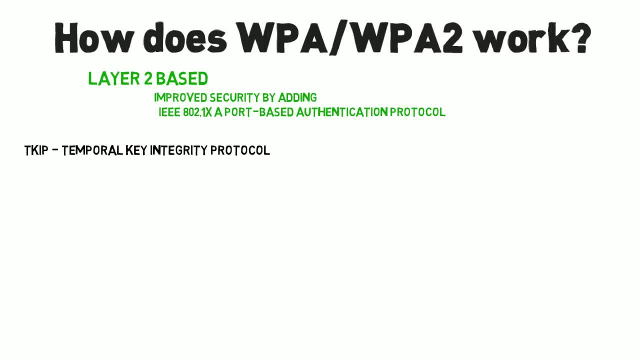 and can be implemented into software with just a driver or firmware update. Cenexonena: torrential ventures in and out of the Web. Carbon District به ретardatvermmor: 2790 일만. enO. Keys are rotated frequently. 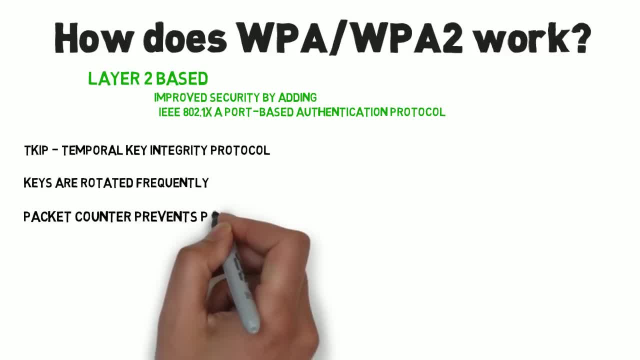 And the Packet Counter prevents packet replay or packet flashing over and Donald Trump, Johnson C subsidized summon classes packet re-injection attacks. WPA provides integrity checking using message integrity code MIC. Although this check some method can be attacked with brute force methods. network traffic is halted automatically for a minute and the 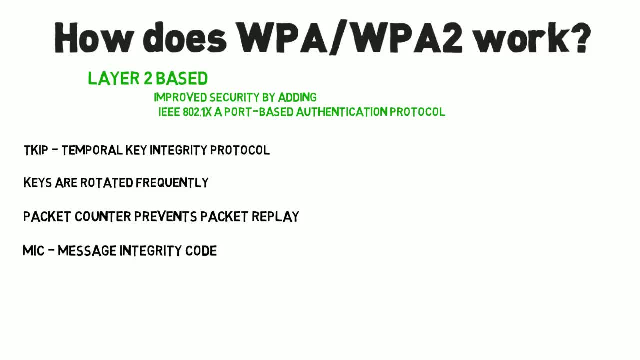 session keys are reset if a WPA based access point detects more than one TKIP MIC failure within 60 seconds. WPA2 uses a new encryption method called counter mode with CBC MAC protocol, CCMP, which is based on a WPA based access point. WPA2 uses a new encryption method called counter mode with CBC MAC protocol, CCMP, which is based on. 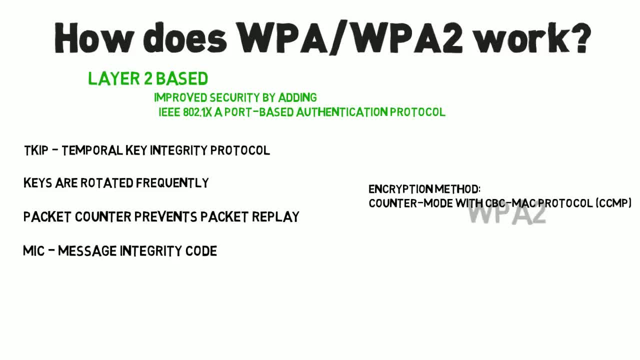 counter mode with CBC MAC protocol, CCMP, which is based on advanced encryption standard AES, a stronger encryption algorithm than RC4.. Both WPA and WPA2 include two authentication modes: personal and enterprise. WPA2 personal generates a 256 bit key from a plain text passphrase. 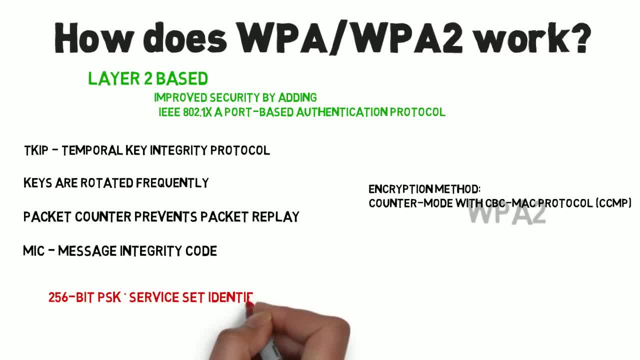 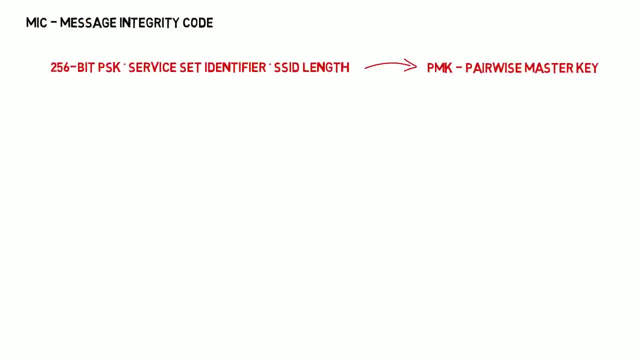 which is called pre-encryption. Both WPA and WPA2 have a pre-shared key, PSK. The PSK, in conjunction with the service set identifier and the SSID length form the mathematical basis for the pairwise master key PMK that is used to initiate a four-way handshake and generate the. 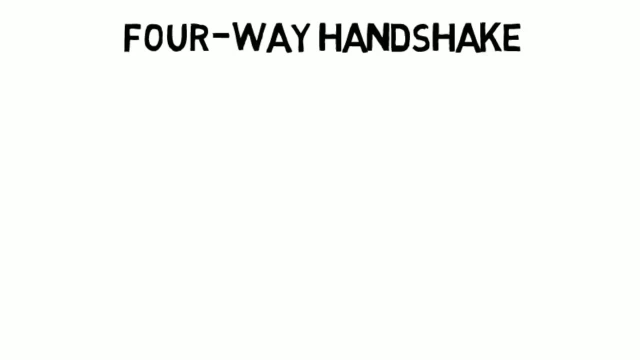 pairwise transient key, also known as PMK. Both WPA and WPA2 have a session key between the wireless user device and the access point. Challenges in WPA2 personnel are the key: distribution and maintenance. The authentication process leaves two considerations. The access point still needs to authenticate. 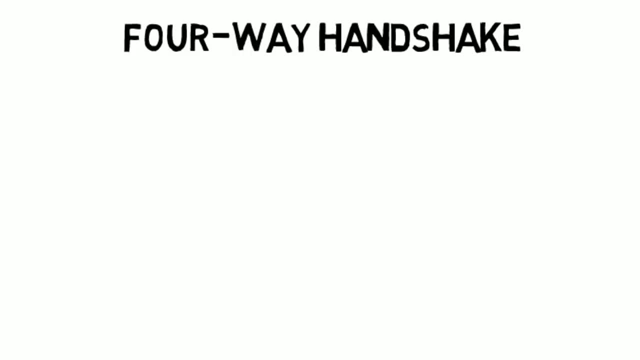 itself to the client and keys to encrypt the traffic need to be derived. The earlier each key is most often used in the current lockout, the more than one key of the handshake is needed to be authenticated. The PAP exchange, or WPA2-PSK, has provided the shared secret key, PMK pairwise master key. 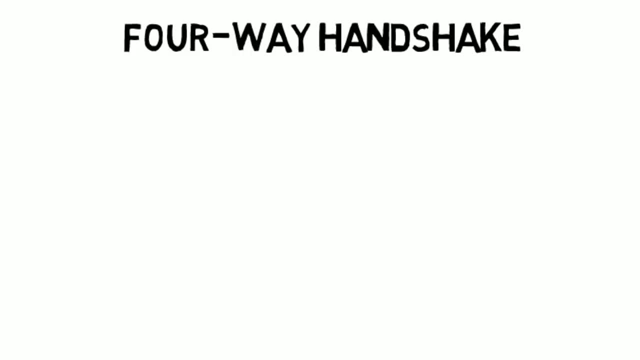 This key is, however, designed to last the entire session and should be exposed as little as possible. Therefore, the four-way handshake is used to establish another key called the PAP key. Theщее key PMK is also used to authenticate the PAP to the earlier the session, then the 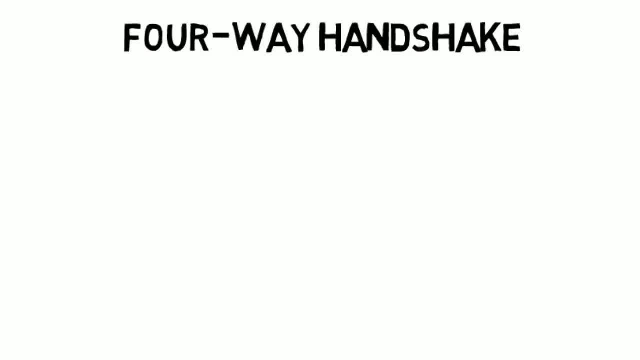 next session in the prior management is used. It is also used to authenticate the PAP key- usingло should be prohibited to enter- and P-T-K pairwise transient key. The four-way handshake, First message A from the authenticator to the supplicant. 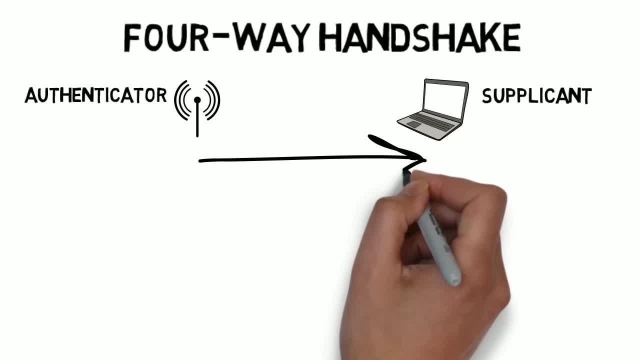 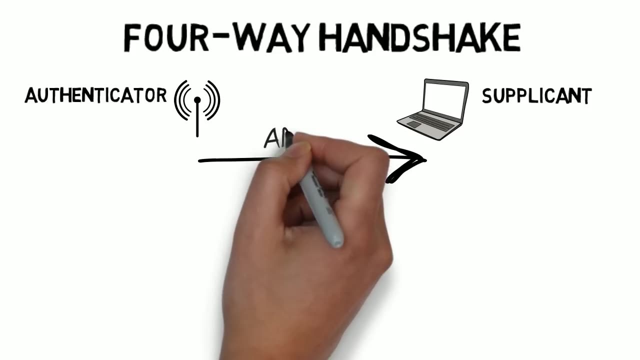 At starting state. no keys are known and therefore no message integrity code M-I-C can be computed. The authenticator uses this message only to send its value of anons to the supplicant. This message is sent without any protection. 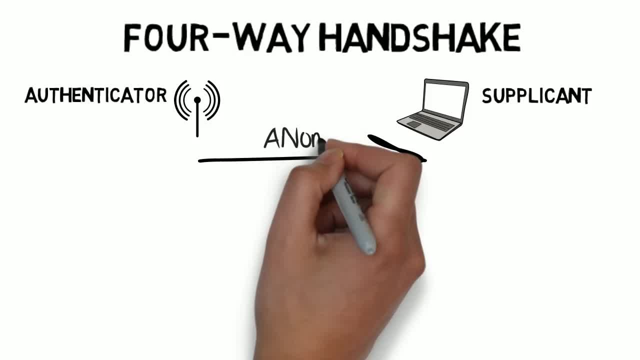 It is not encrypted and there is no M-I-C. This is the only key message that is ever sent without the M-I-C bit set to 1.. If any of the fields in this first message is not set according to the standard. 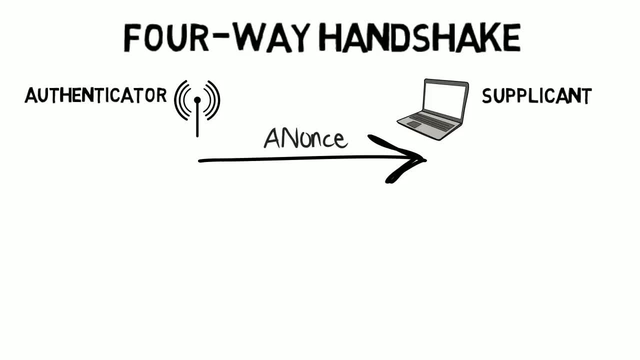 the supplicant should discard the message. The only fields which can be modified according to the standard are the replay counter or the anons Change. Changing the replay counter can only result in a message rejection and is therefore pointless. Any changes to the anons value will be recognized in message B. 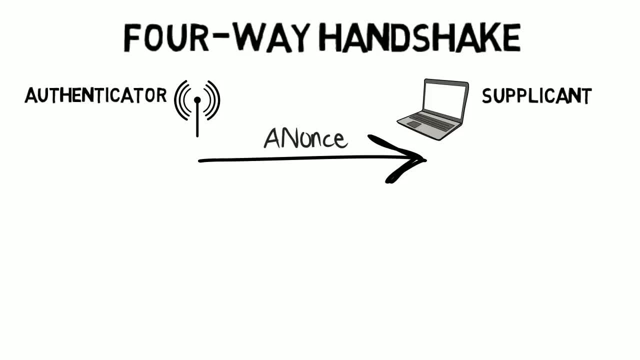 because the temporal keys computed by the supplicant form, the corrupted anons value, would be invalid. In such a case, message B would fail the M-I-C test and be discarded. The fact that message A is unprotected does not compromise security. Second message B from the supplicant to the authenticator. 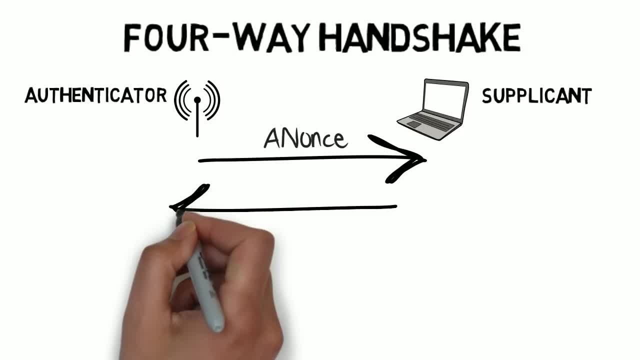 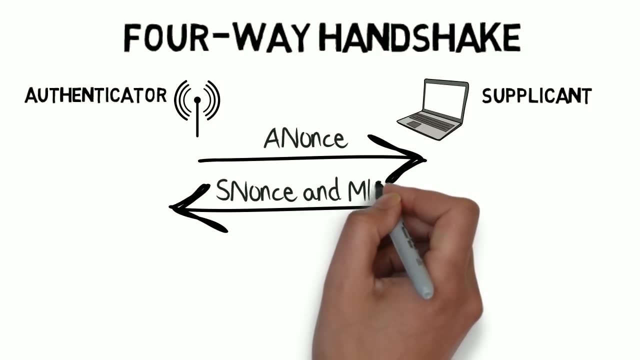 After successful delivery of the first message, the supplicant has a copy of anons and generates its own value of esnons. It is then able to compute the transient key. Next it prepares to send message B to the authenticator. This message contains an M-I-C value and thus proves 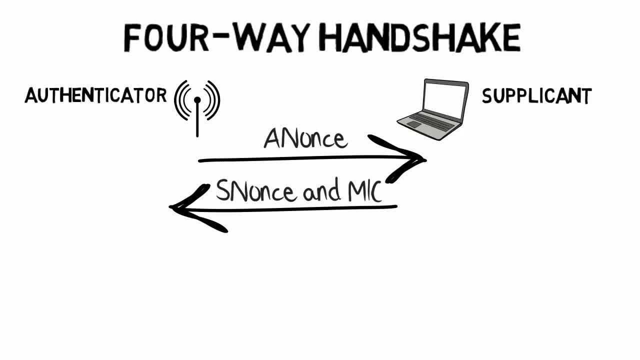 that the M-I-C value is the M-I-C value. of the M-I-C value, The supplicant knows the pairwise master key P-M-K. The fact that the descriptor type field is 1 indicates that the M-I-C value should be computed using a logarithm. 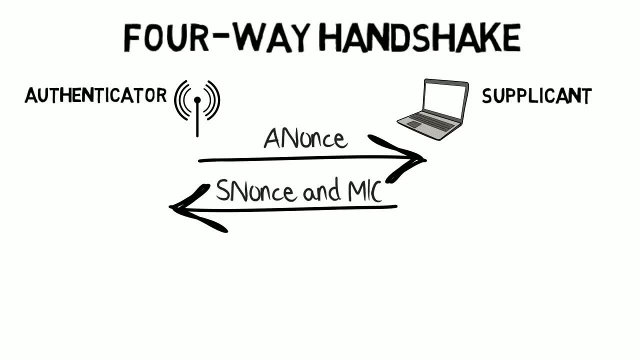 called HMACMD5, which produces a 16-byte M-I-C value. The M-I-C calculation is performed over more than just message B. It includes all the bytes from EPAL in the header up to and including the key data. Third message C: from the authenticator to the supplicant. 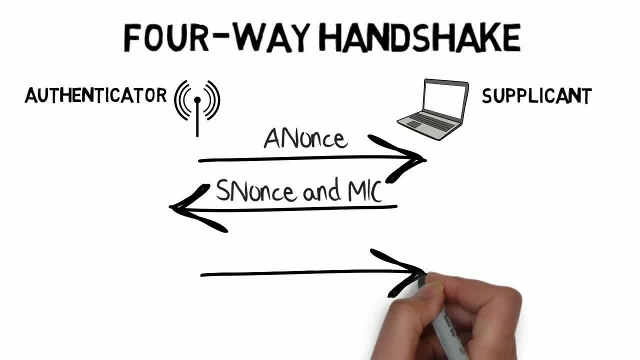 When message B is received by the authenticator, it is able to extract the value of esnons because the message is unencrypted. The authenticator then has all the information to compute its copy of the temporal keys. After this is done, the pairwise key distribution. 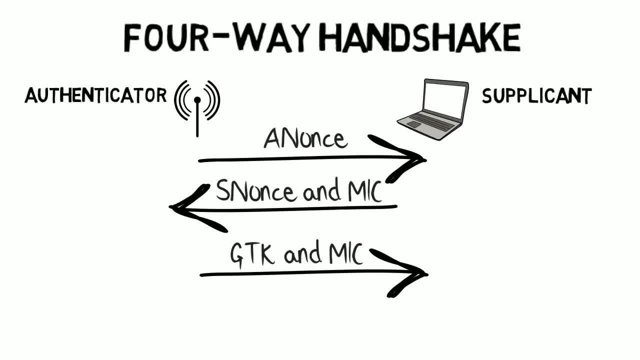 is effectively completed. However, the remaining message exchanges. messages C and D are used to ensure that the keys are put into effect in a synchronized way. Message C serves two functions. First, it verifies to the supplicant that the authenticator knows the P-M-K. 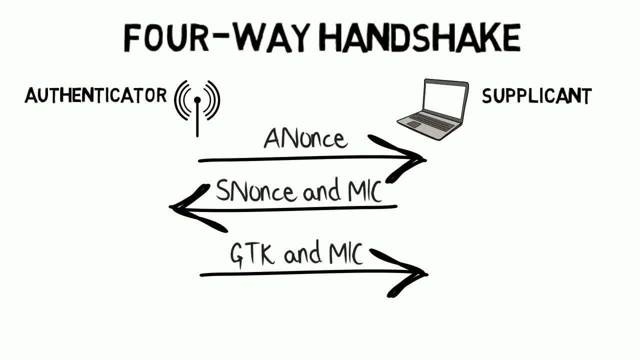 and is thus a trusted party. Second, it tells the supplicant that the authenticator is ready to install and start using the data encryption key. This authorizes a message through the key theme and opens the key key. The authenticator does not actually install the keys until it has received message D. 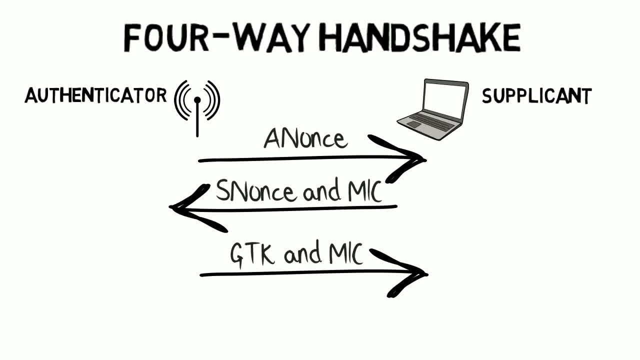 Note that if a re-transmission of message C is needed due to failure to get a response, the re-transmission should be a copy of the original unencrypted transmission. Last transmission D from the supplicant to the authenticator: This final message verifies to the authenticator that the keys are about to be installed. 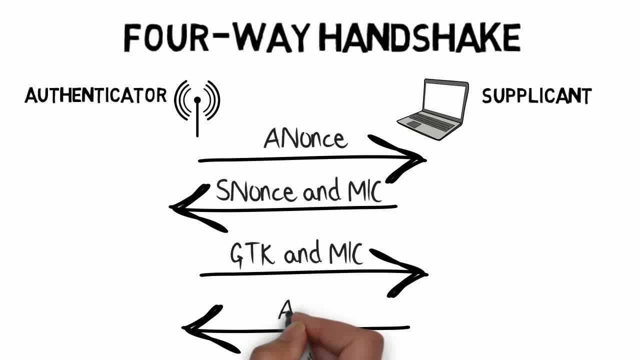 There is nothing surprising or new. when the supplicant has received message D Key is entered into the key theme and the P-M-K is completed. the setting for this message, which is similar to message B, but without the key data field. 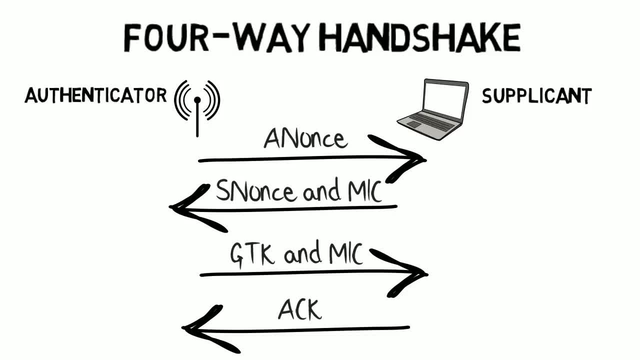 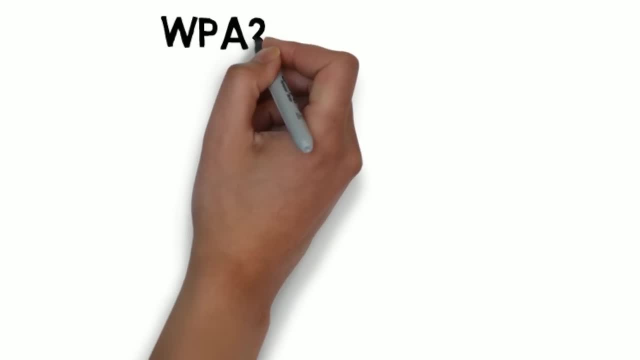 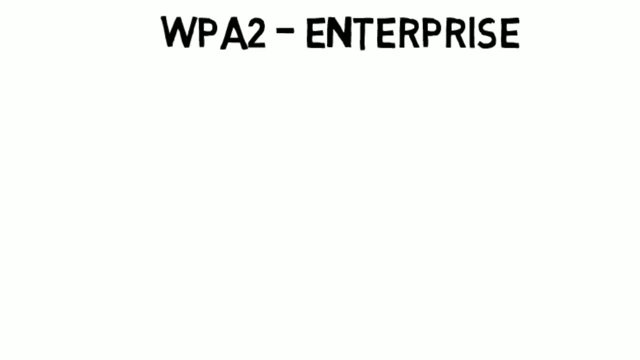 The secure bit is not set until the four-way handshake is successfully completed and both supplicant and authenticator have installed the keys. This does not happen until message D has been received and decoded successfully. WPA2 Enterprise addresses concerns in respect to distributing and managing static keys and controls access on a per-account basis. 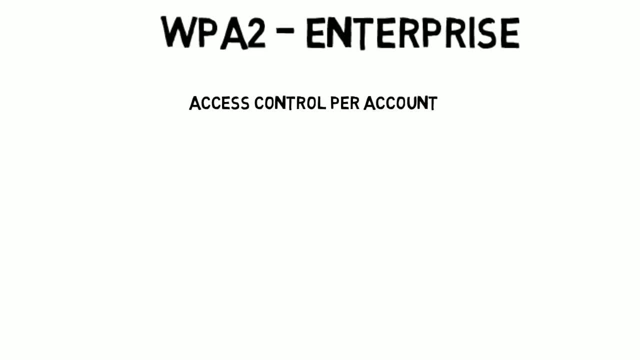 by integrating most organizations' authentication services. Therefore, credentials like username and password certificate or a one-time password are necessary to authenticate the client. on the authentication server, The access point or wireless control controller monitors the connection and redirects authentication packets to the appropriate